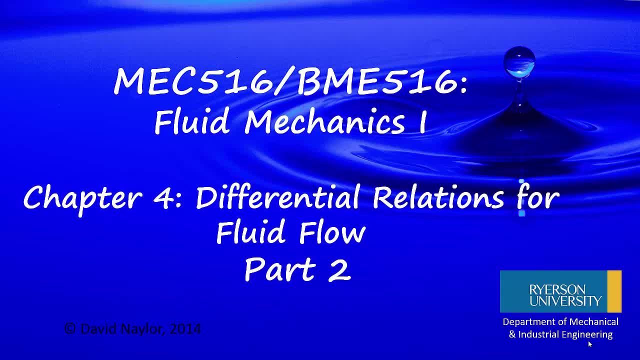 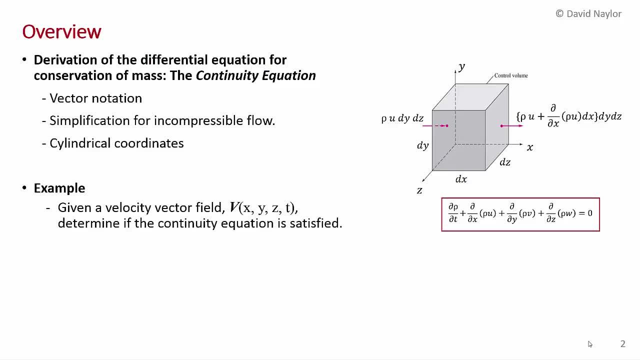 This is chapter 4, differential relations for fluid flow, part 2.. In this video I'm going to derive the differential equation for the conservation of mass. As you learned in the previous video, this is called the continuity equation And in the previous video I showed you. 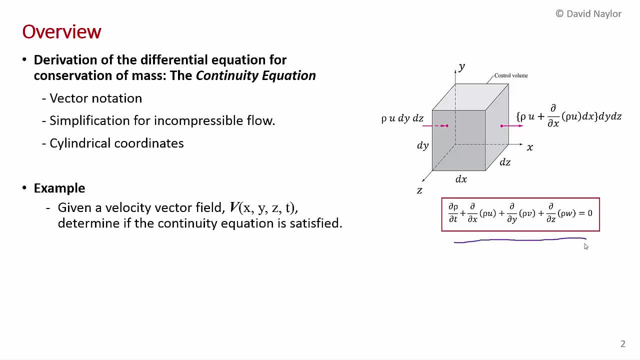 the result. The result is shown here over on the right, so that's what we're going to derive. Then, once we've completed that derivation, I'll show how you can express this in vector notation, which is important for fluid mechanics analysis. Then I'll show how you can simplify the continuity. 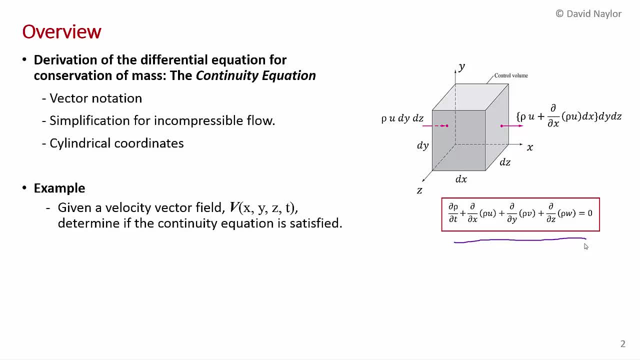 equation, the general form of the continuity equation for incompressible flows where density is a constant, And then we'll talk about how to derive this equation in cylindrical coordinates. The use of cylindrical coordinates is very important. The use of cylindrical coordinates is important when you're analyzing sort of naturally cylindrical objects like flowing pipes. 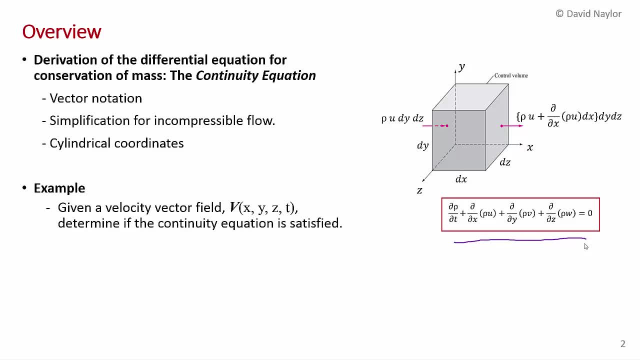 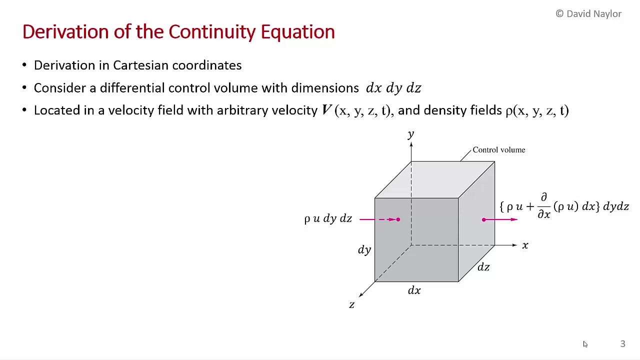 And then we'll end with an example where I give a velocity vector field, V, and I'll show you how to determine if that vector field satisfies conservation of mass or the continuity equation. So I'm going to start with the derivation of the continuity equation in Cartesian coordinates. So, as shown in the diagram, we're going to 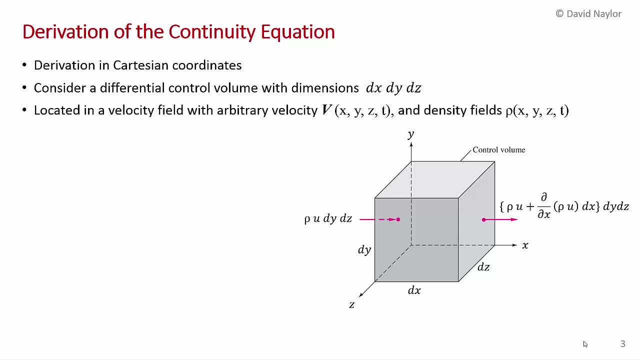 consider a differential control volume with dimensions dx, dy, dz, And this control volume is assumed to be located in an arbitrary velocity vector field V of the three coordinates x, y, z and time, And density also can vary with x, y, z and time. 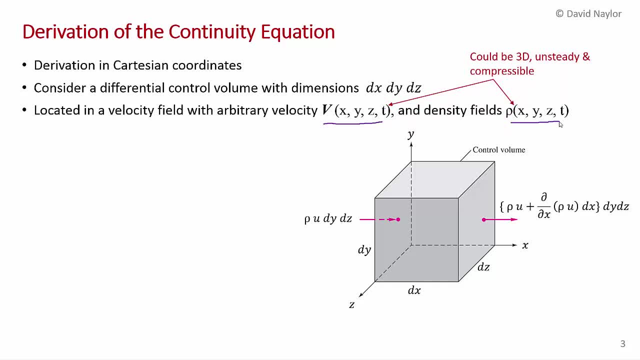 So at this point we're not making any simplifications. The flow could be fully three-dimensional, it could be unsteady and it could be compressible. So we start by considering the mass flow rate into this little differential control volume in the x direction. Now you remember that mass flow rate is rho times, velocity times. 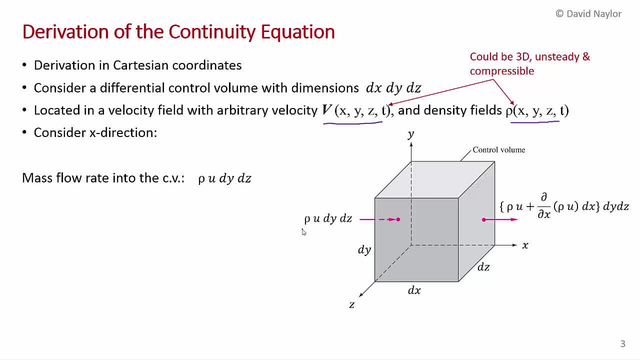 area, And so that's what we have. We have density times, the velocity in the x direction times, the area y, dz is the area of this face here. So that's the mass flow rate in, For the mass flow rate out at x plus dx, we do a little. 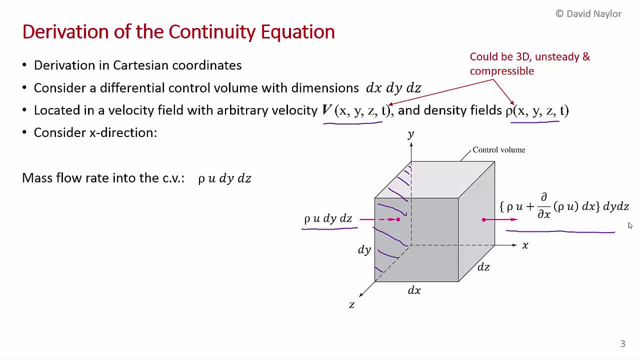 Taylor series. here We take rho u and then dA here is outside the brackets And then dy by dx of rho u, dx, The dx's will cancel. it'll give you the small change in rho u in that direction. Now of course there are higher order terms And let me rewrite it down here: The mass. 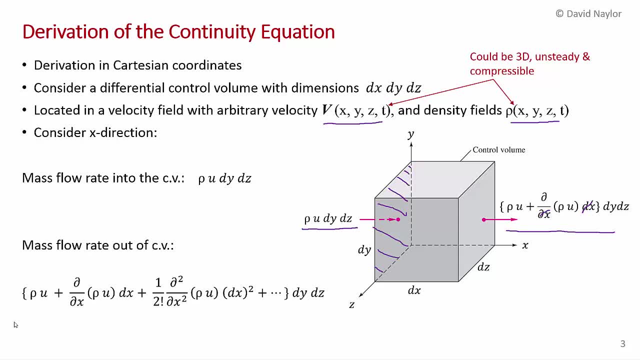 flow rate out of the control volume. I've rewritten it here, the term rho u and then dy by dx of rho u, dx, And of course there would be higher order terms here There'd be 1 over 2 factorial. the second derivative in the x direction: times rho u times dx squared. 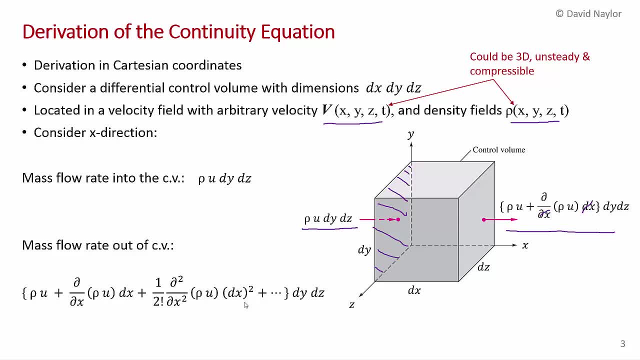 and then 1 over 3 factorial, the third derivative, et cetera, et cetera. But when you're doing this kind of analysis, when you let, ultimately, when you let dx go to 0, and you're considering flow at a point, 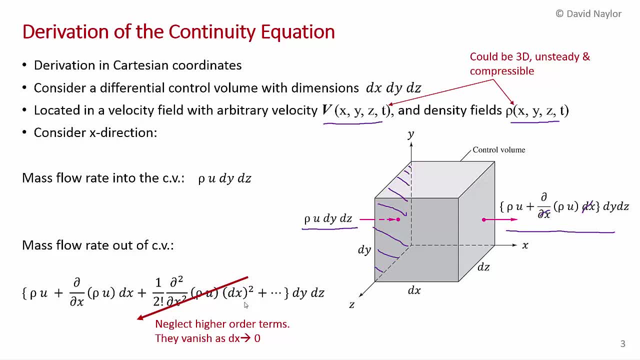 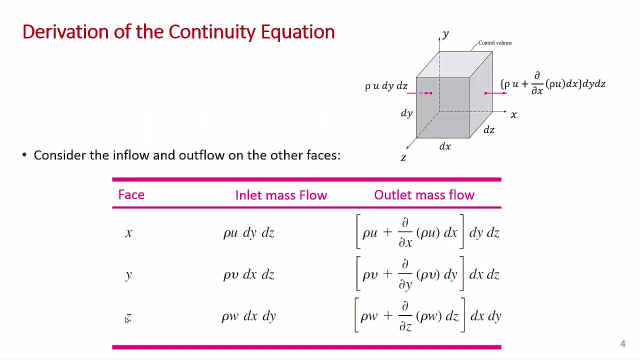 these higher order terms vanish much more quickly than the linear terms, And so we're just left with the linear derivative term here. So that's the x direction. Now you can do exactly the same thing in the y and z directions. You can look at the mass flow. 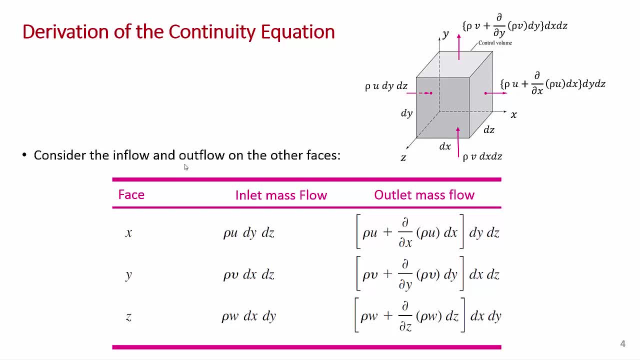 in and I've written the terms here for the y direction, So rho v this time times the area dx, dz. So now we're talking about this area here, And then I've done the same thing at the top here. I've taken the partial derivative in the y direction of rho v dy and added it. 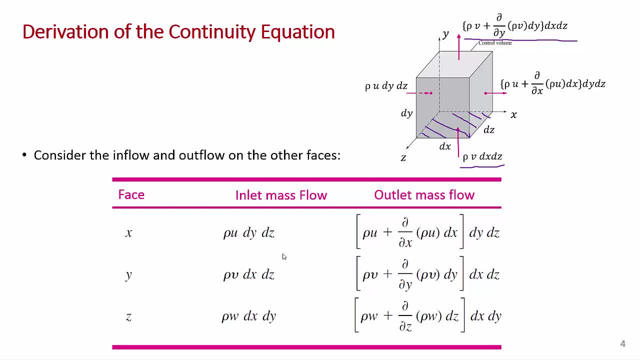 onto rho v, And so what you get is the inlet term in the x direction, the partial derivative term in the y direction of rho v, the outlet term in the x direction. We just showed the inlet term in the y direction, the outlet term in the y direction, And you can do exactly. 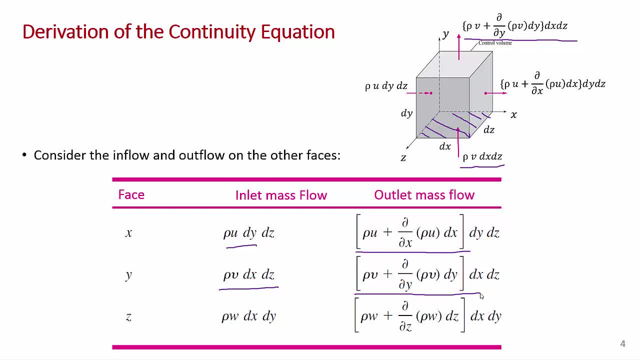 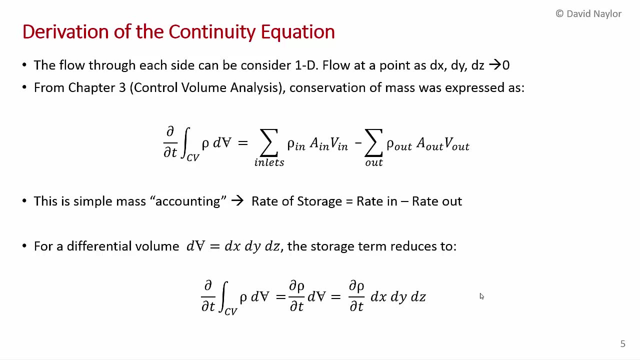 the same thing in the z direction. It's very easy, So now it's just a matter of doing some fairly simple mass flow accounting and making sure that these all balance. Now I should point out that the flow through each side in this little control volume can. 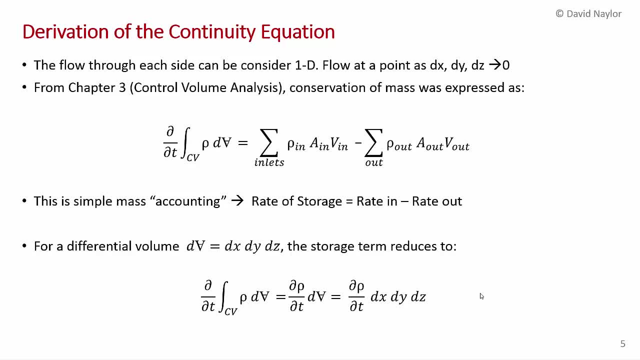 be considered one dimensional because ultimately we're going to shrink this, we're going to shrink this control volume to let dx, dy and dz go to zero. So we're considering flow at a point, So you don't need to worry about the variation of the flow across each face. 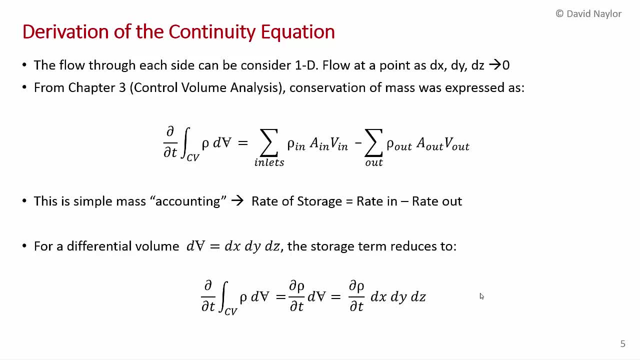 From chapter three. in our control volume analysis we showed that conservation of mass can be expressed as: the rate of storage in the control volume equals the rate at which mass flows in, minus the rate at which mass flows out. This is just simple accounting, Remember. so rate of storage equals rate in minus rate. 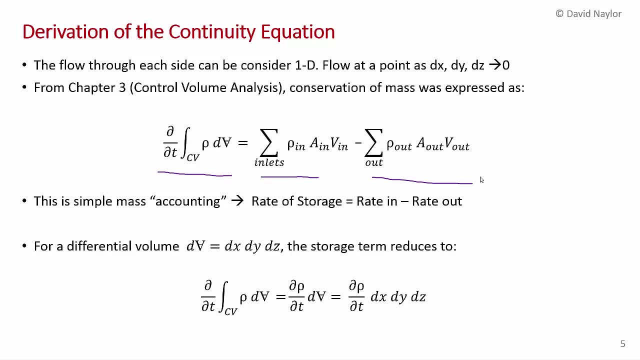 out. you can do the same thing on your bank account. We talked about that. So we have the inlet and the outlet terms. I just need to talk a little bit about the storage term here. This storage terms here we, when we derived this, we derived it for. 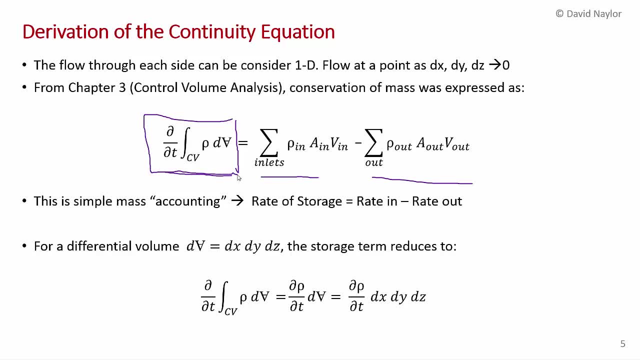 a finite sized control volume. but right now we're doing an analysis on a differential volume that we're going to let Short desired Из, short desired Wir, short desired Id, short desired Ad shrink to zero. So you really, as I mentioned, the properties are constant over that differential. 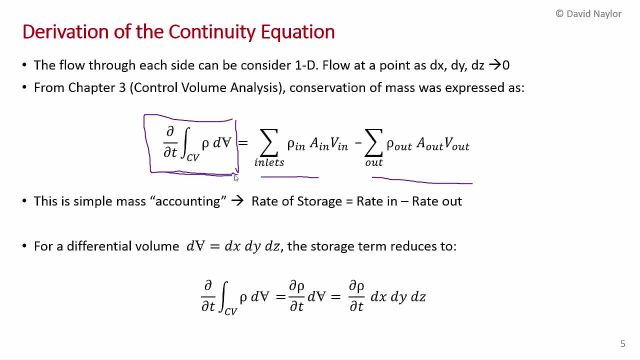 volume as the differential volume shrinks to zero, which is what we do in calculus. So we don't really need to perform that integration. We can just express this as dy rho, dy, t times the incremental volume, and the incremental volume is dx, dy, dz. So we have our storage. 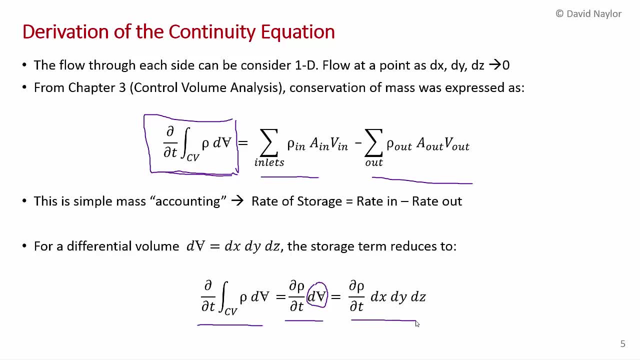 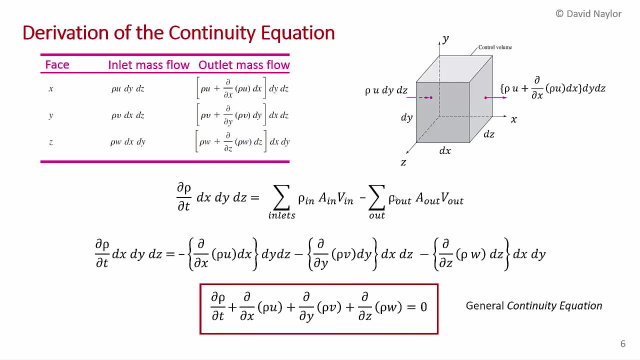 term here, which is the partial derivative of density times the incremental volume. Now we can substitute in, and that's what I've done. on the next slide I've reproduced the table- Here's the table that we had- and I've reproduced the conservation of mass. 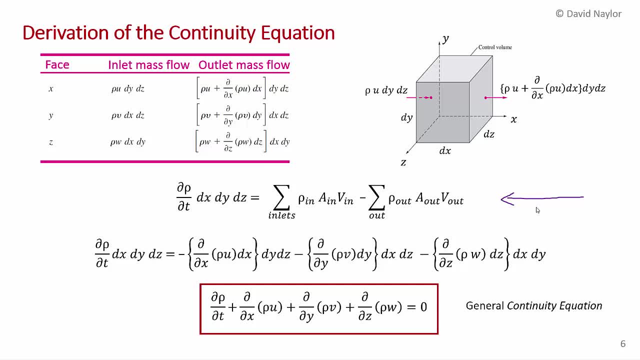 equation for a control volume. Now what we do is we substitute in the inlets and the outlets. but there's a little simplification been made here, If you notice that the rho u dy dz- here this term really cancels with this term. So in and out And 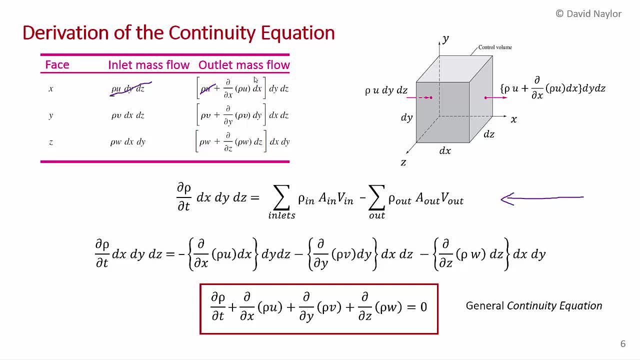 what we have here is in minus out, so what you're going to retain is the negative. this term times the negative and, similarly, we're going to retain the negative of this term because it's in-minus-out, And we're going to retain the negative value of this term. 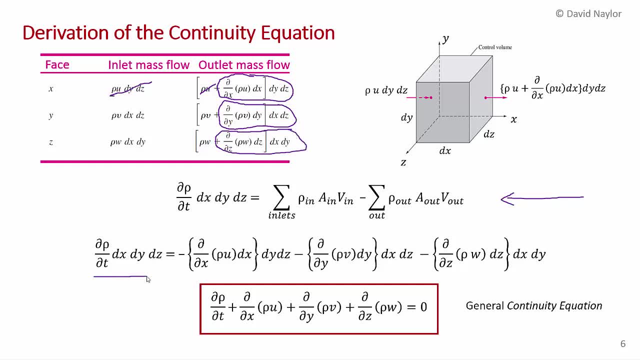 And so that's what you want. So I hope that's helpful. Thanks for watching. what you have is the rate of storage. here equals these three terms added up, but they're negative because it's the mass flow rate in minus the mass flow rate out. So now you can see that each one of 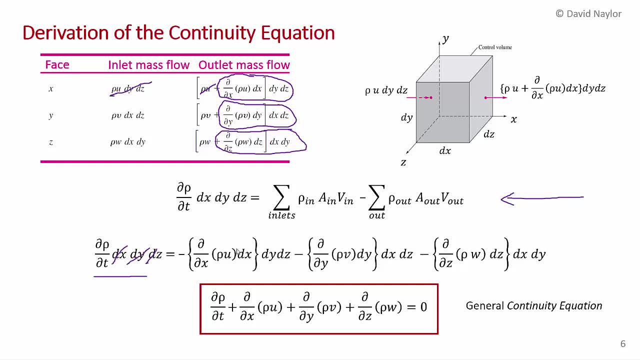 these terms has dx dy, dz. So you can get rid of dx dy, dz And we end up with the final result at the bottom, which is the general continuity equation. And that's the final result. It's a very 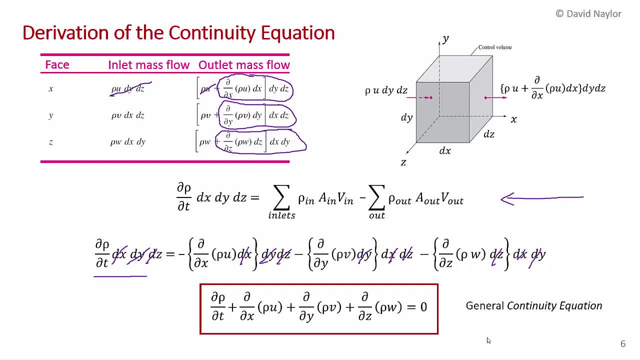 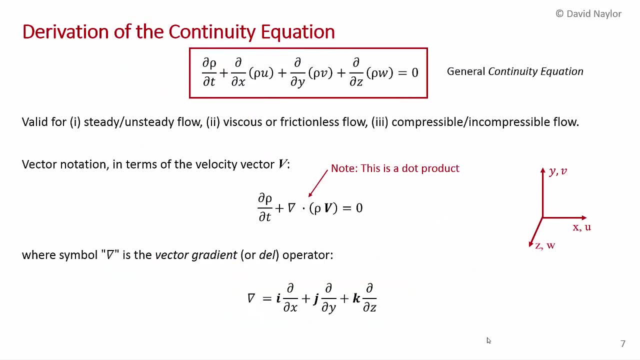 simple derivation. It's worthwhile learning how to do this and understanding the result, So I've rewritten the general continuity equation here up on the next slide. I wanted to emphasize that this applies for both steady and unsteady flows, Of course. if it's steady, then the time 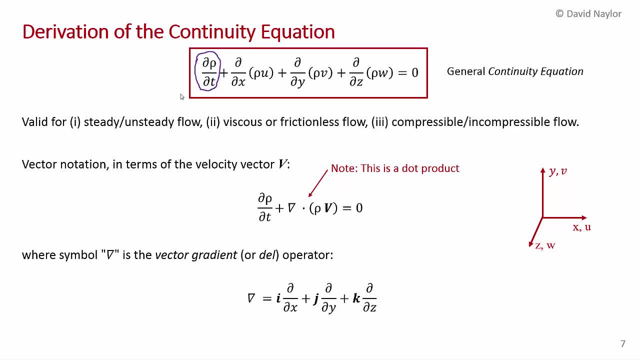 derivative goes to zero. So if it's steady, then the time derivative goes to zero. So if it's steady, zero, so this term goes away. This is the general form. It's applicable for flows that have viscosity or do not have viscosity, so inviscid flows or viscous flows, It's also applicable. 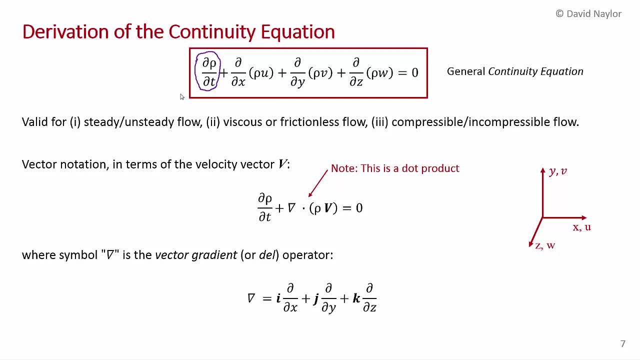 for compressible or incompressible flows In the derivation we have left density as a function of x, y, z and time. What I'd also like to do is talk about vector notation, because vector notation is widely used in fluid mechanics and fluid dynamics analysis. So you'll often see in 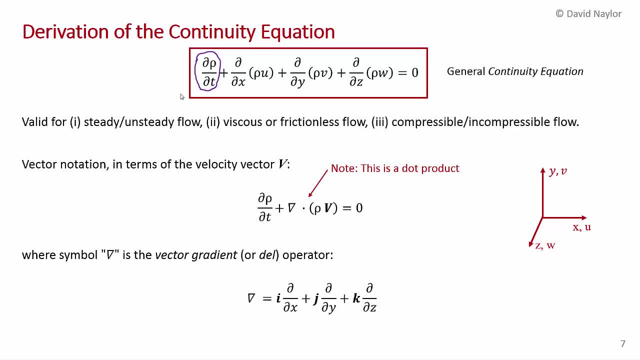 textbooks and in papers, the continuity equation written in vector notation, And so I've written it here in vector notation. We have the partial derivative of density with time, and then I want to introduce- you may have seen this before- this upside down triangle, if you like, It's called. 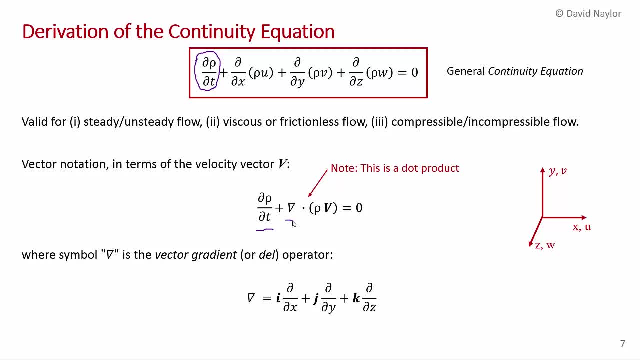 the vector gradient, or delta, And so what we're going to do here is we're going to use the delta operator, And the delta operator is just die-by-day x in the i direction plus die-by-day y in the j direction, die-by-z. 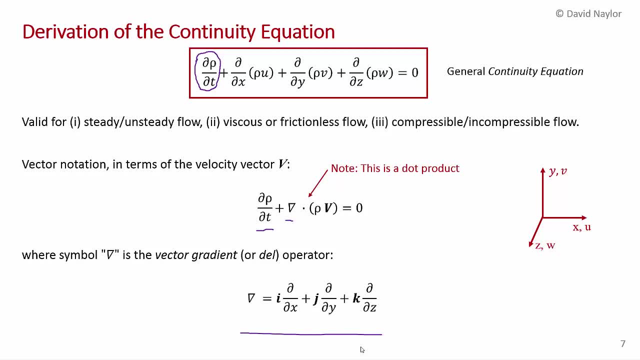 in the k direction, of course, where i, j and k are the unit vectors in the x, y and z direction. So you can see, if you note that this little dot here is actually a scalar product or a dot product, that if you apply this operator to this row v, where v is the dot, then you're going to 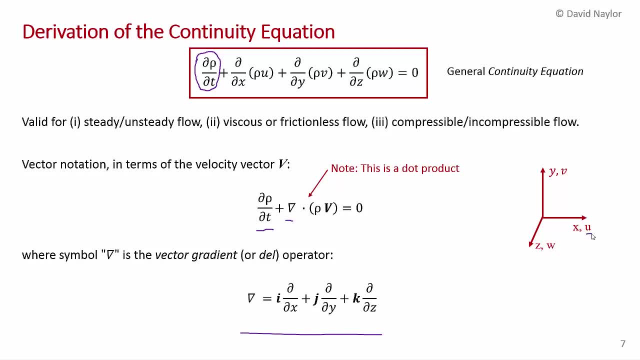 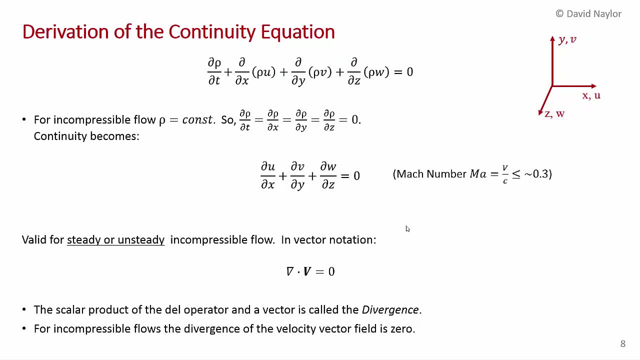 see that v has the three components u in the i direction, v in the j direction and w in the k direction. you would recover the general continuity equation. So it's worth learning about and understanding the del operator. Here again, I've written the general continuity equation at the top. That's our result, that we're 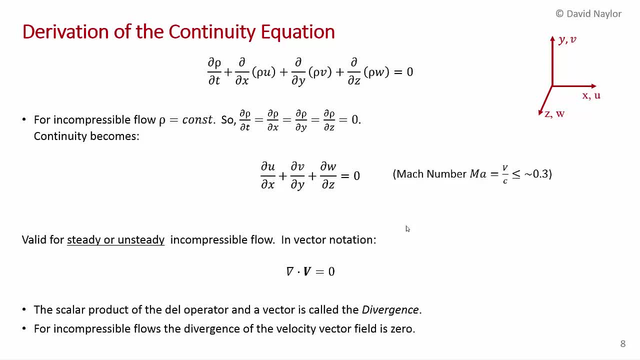 working with. So what we're going to do is simplify this for incompressible flows. So when you have an incompressible flow, that means that the density is a constant. So density doesn't vary spatially, it doesn't vary in the x, y or z direction and it doesn't vary in time. So with that, 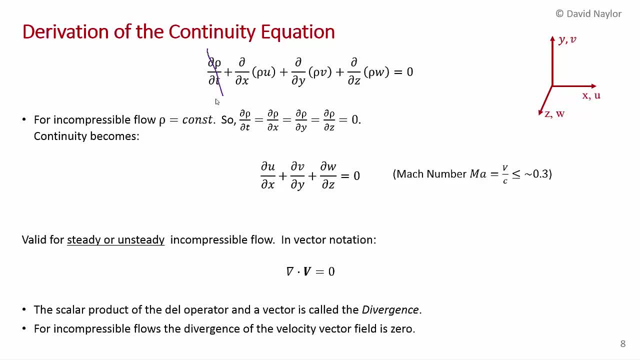 simplification, you can get rid of di rho, di t and you can bring density outside of the derivative. If you do that in all three cases, then you can cancel density And you just end up with. this is the incompressible form of the continuity equation. 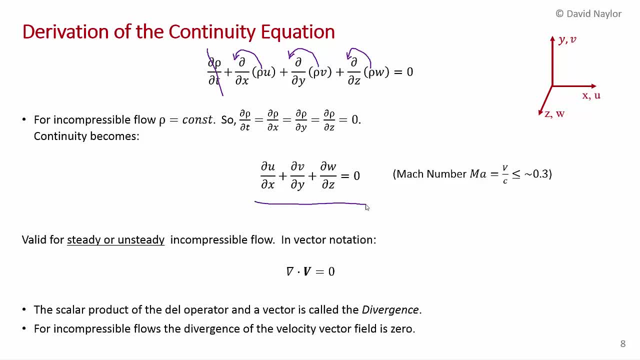 It's di u by di x plus di v by di y plus di w by di z. So the rate of change of the x component of velocity in the x direction, plus the rate of change of the y component of velocity in the y direction, plus the rate of change of the z. 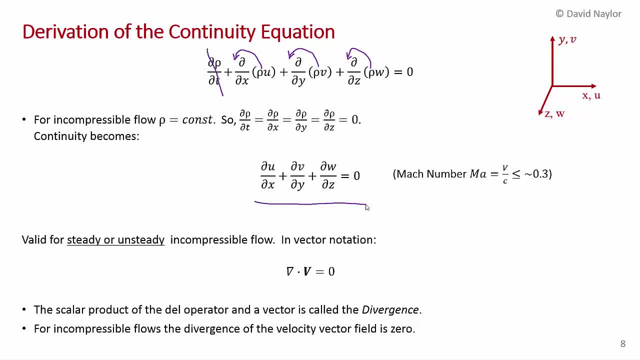 component of velocity in the z direction all have to add up to zero when you have an incompressible flow, And of course that's the equation you would use for liquids for most conditions. For gases, you have to worry about compressibility. 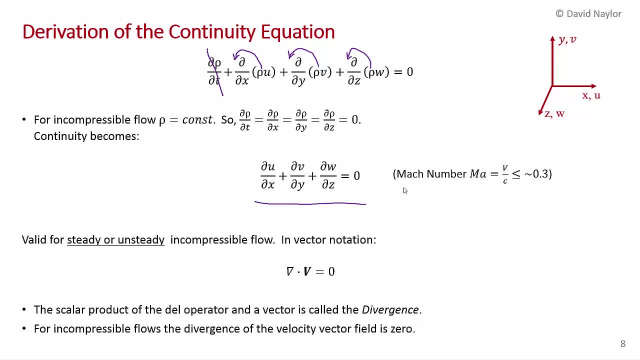 And we talked about this earlier- that typically you can apply or you can use the incompressible assumption when the Mach number is less than 0.3, where the Mach number is the velocity over the speed of sound in the gas, And we talked about this in previous videos. 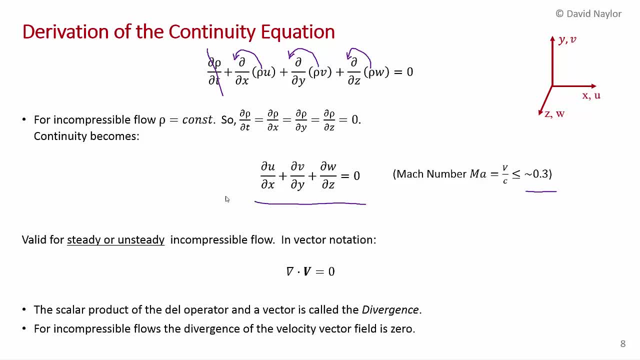 So what's a little bit surprising about this equation is that you haven't made the assumption of steady flow. So this equation is valid. this incompressible equation is valid for steady or unsteady flows, Incompressible flows In vector notation. now this just becomes that del dotted into the velocity vector equals zero. 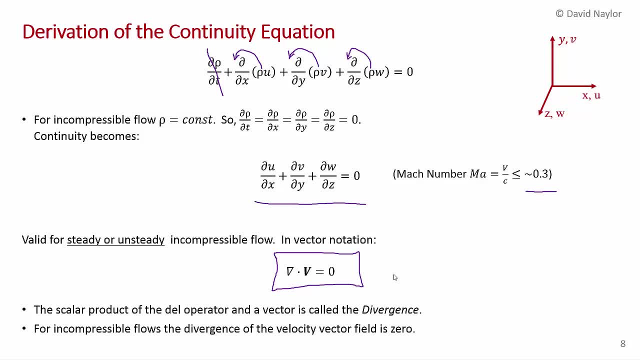 In mathematics this scalar product of the del operator and a vector is zero, so that's a little bit surprising. So what's a little bit surprising about this equation is that you haven't made the assumption of steady flow, and a vector is called the divergence, and so in fluid mechanics we say that in incompressible. 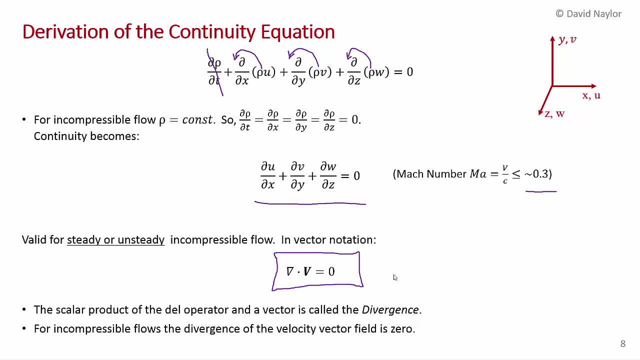 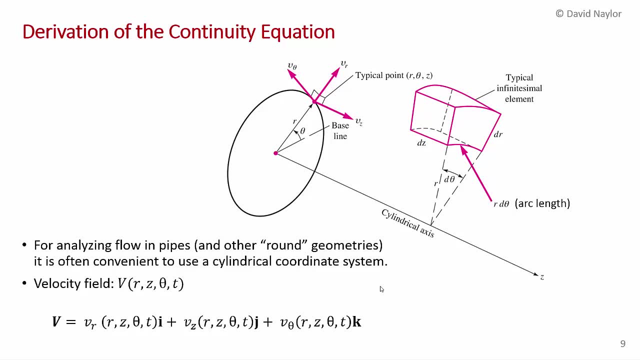 flows, the divergence of the velocity vector is zero, and that's what this equation expresses. So that was the derivation in Cartesian coordinates. now, as I mentioned, for analyzing flow in pipes and other sort of naturally round geometries, it's often convenient to use a cylindrical 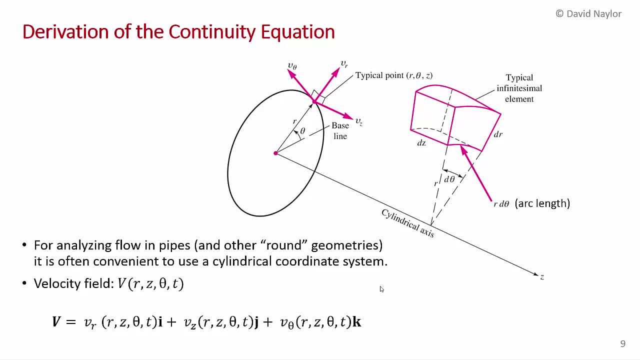 coordinate system. so instead of x, y, z, now we have r, z and theta. so some radius, some distance- z axial distance- and some angle- theta. So a typical point would be defined by three coordinates: r, theta and z. and now we have 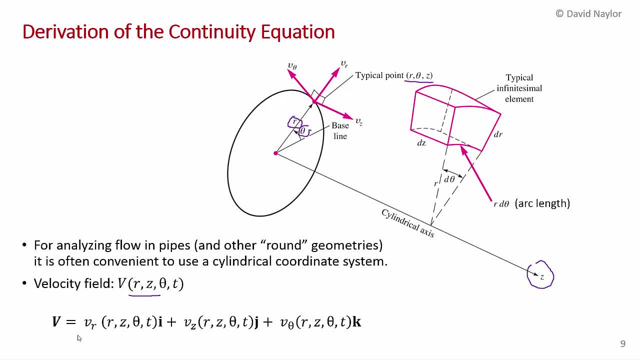 three velocity components- vr, vz and vz- And they're shown in the diagram here. Now this seems complicated, but it actually is not very complicated to derive. I'm not going to re-derive the continuity equation for this situation, but I'm just 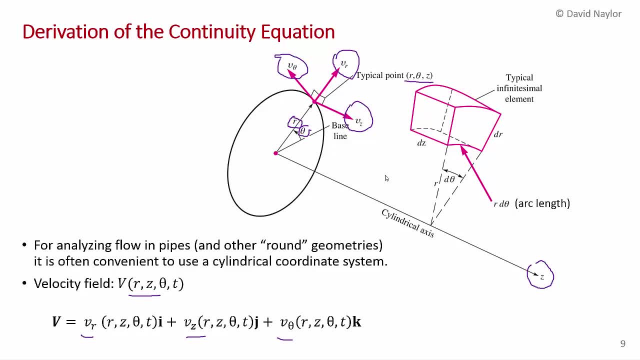 going to give you a little hint. You can complete the rest of this on a piece of paper. it takes about a half a page to do this, If you consider I'm going to show you the hardest one. so if you consider a little cylindrical. 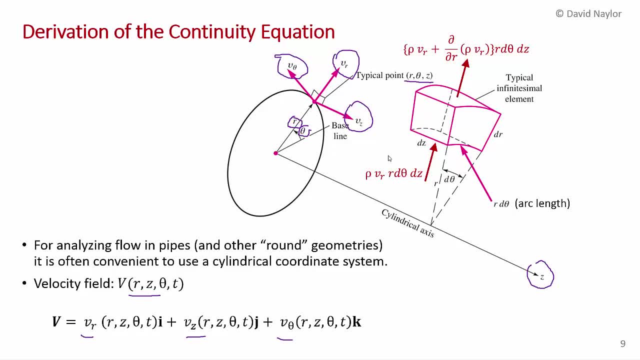 element now. Now, if you do the mass balance, what you've got to consider- and here's the little trick here- is that this distance here is r d theta, remember that's arc length. and so now, if you're considering the r component of velocity, you have rho vr. now you want 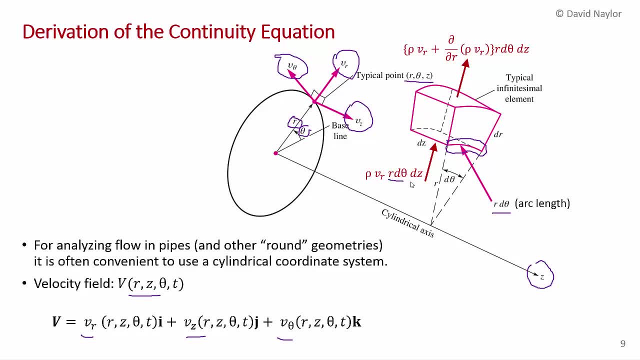 to get times dA. now dA is the arc length, r d, theta times d, z. and then you do exactly the same thing at r plus dr. You express this little linear derivative: Okay, So rho vr times d by dr of rho vr and then times this here, which is dA. 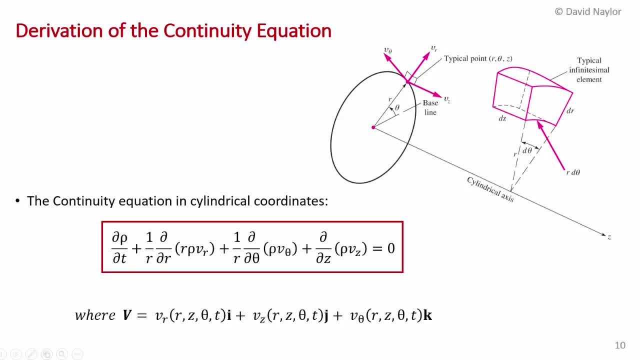 From here it's pretty easy to complete the rest of the analysis. You can try this as an exercise, if you want, and then what you get is the continuity equation that I've shown here. So it's 1 over r d by dr of r rho vr. 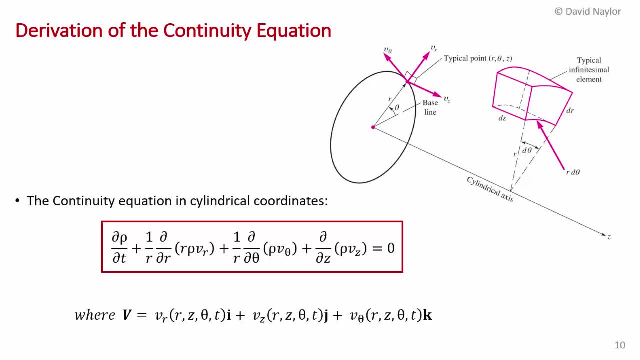 Plus 1 over r d by d theta, rho v theta. plus d by d z of rho v z. It looks more complicated, but it's actually not very complicated to derive at all And that's very useful and we will be using it when we look at fully developed flow in. 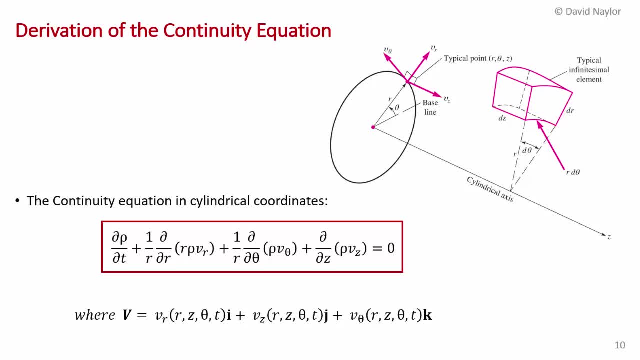 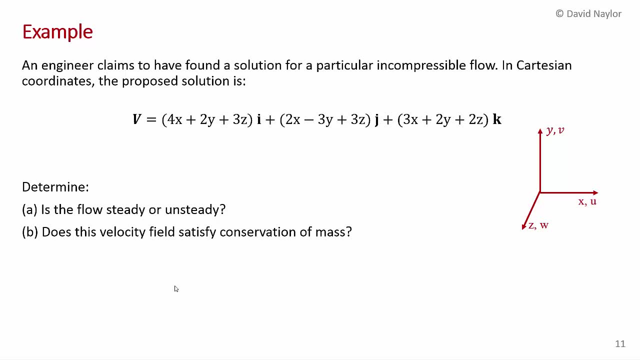 pipes. So I'd like to end with just a simple example. An engineer claims to have found a solution. It's a solution for a particular incompressible flow, and in Cartesian coordinates the proposed solution is given here, where we have v equals 4x plus 2y plus 3z in the i direction. so 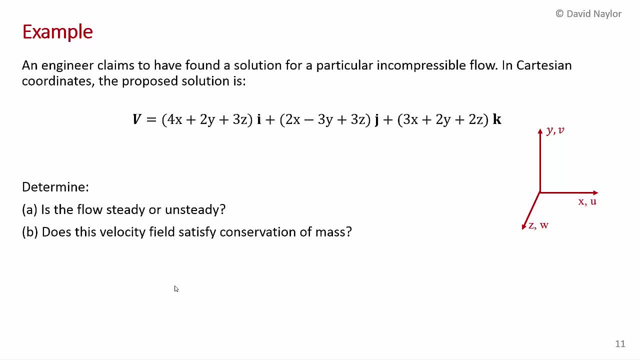 in the x direction, 2x minus 3y plus 3z in the y direction or in the j-hat direction, 3x plus 2y plus 2z in the k or z direction, And you're asked to find a solution. 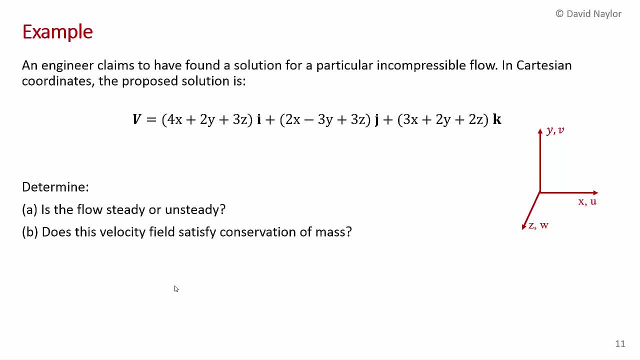 You're asked to find out: is this flow steady or unsteady, and does it satisfy conservation of mass? In other words, does it satisfy the continuity equation? So these three components here are u, v and w, And so you can see answering the first question: is it steady or unsteady? you might pause. 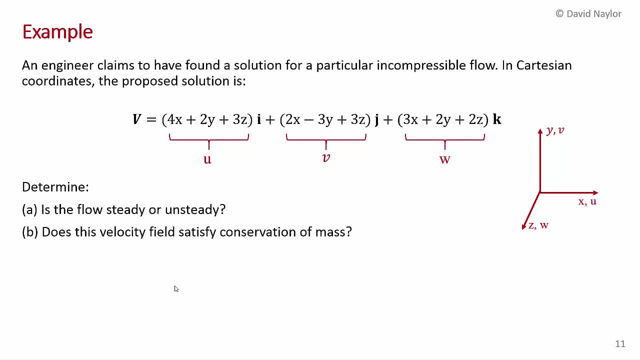 the video and think about this for a moment. So I'll give the answer. The flow is steady. You'll notice that the flow is steady. Notice that u, v and w- there's no time, there's no function of time. 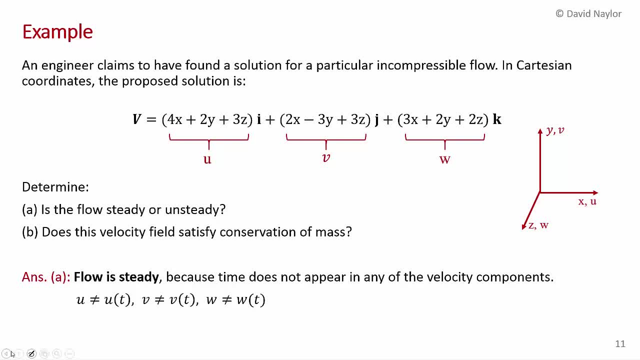 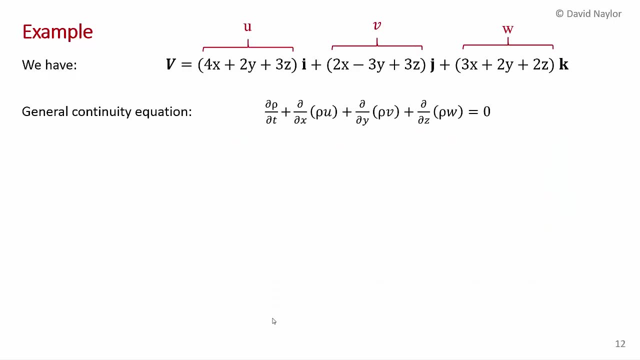 Because time does not appear in the velocity components you have. u is not a function of time, v is not a function of time and w is not a function of time. So we have a steady flow. There's no time dependence. For the next question, as to whether it satisfies conservation of mass, we need to show that. 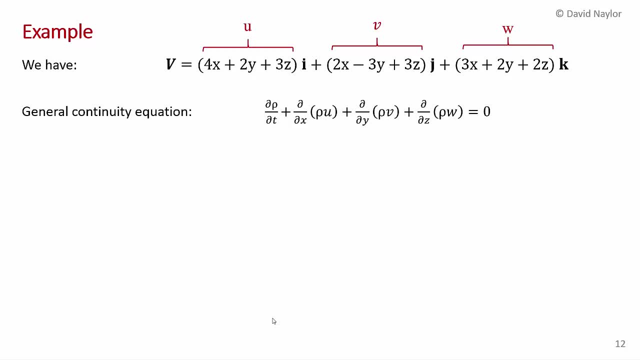 this equation does or does not satisfy continuity, And so I've rewritten the velocity vector that we're given in the problem statement, and reminding you that we have the u, v and w components here in the i, j and k direction. So what we're going to do is apply the general continuity equation. 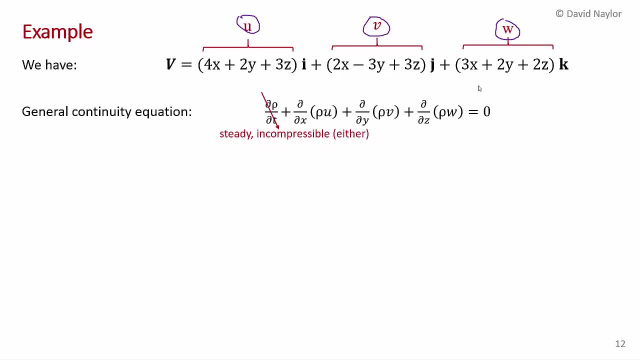 I'd start from this every time, if you like. You're told in the well, we just determined that the problem is steady so we can get rid of d rho vt. But it's also income, You're told in the problem statement. 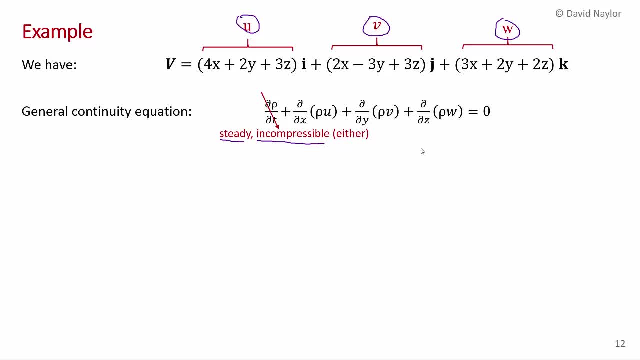 That it's incompressible. So if it's either steady or incompressible, that term goes. It doesn't require both. So now we can simplify this equation for incompressible flow and we just end up with di, u, di x plus. 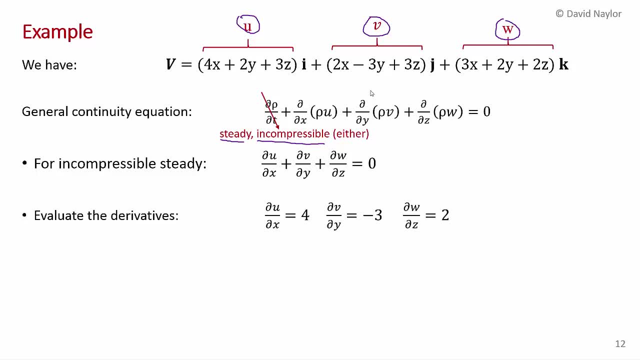 di v di y plus di w di z equals 0.. Now we can evaluate the derivatives, noting that u is 4x plus 2y plus 3z, So di u di x is just 4.. Di v di y is going to be minus 3.. 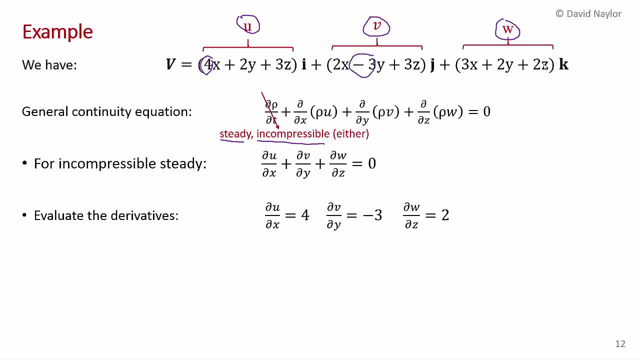 And di w di z is going to be 2.. So we substitute those back into here, right? That goes into there, that goes into there, and that goes into there, and we get 4 minus 3 plus 2, 1, which equals 3..